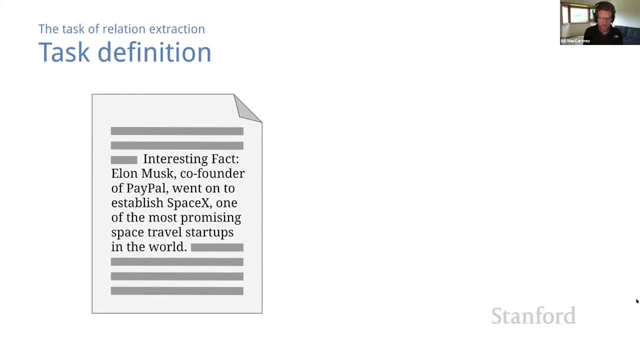 We want to be able to start from a document like this- This could be a news story or a web page- and extract relational triples like founders PayPal- Elon Musk and founders SpaceX- Elon Musk. Next, we find this document and we want to be able to extract it from the original document. 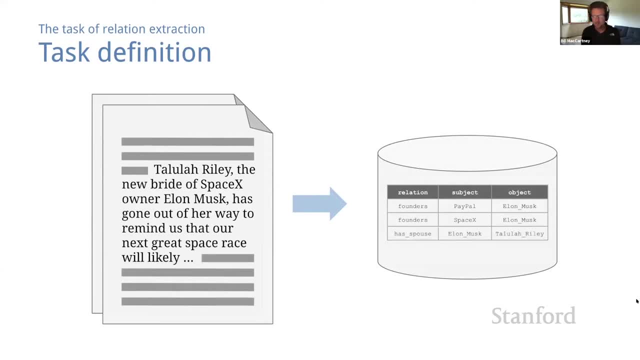 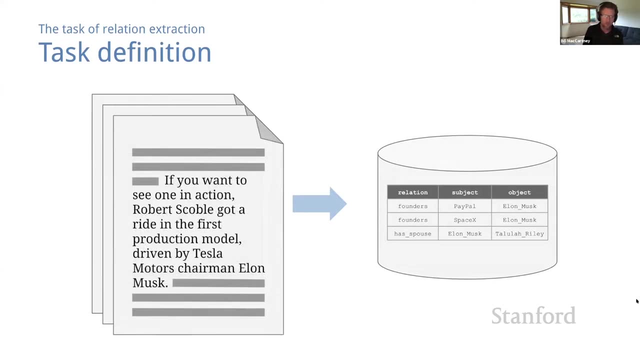 Next, we find this document and we want to be able to extract it from the original document. We use it to extract has-spouse: Elon Musk, Toulouse Riley. We keep reading another document And we want to extract worked-app: Elon Musk, Tesla Motors. 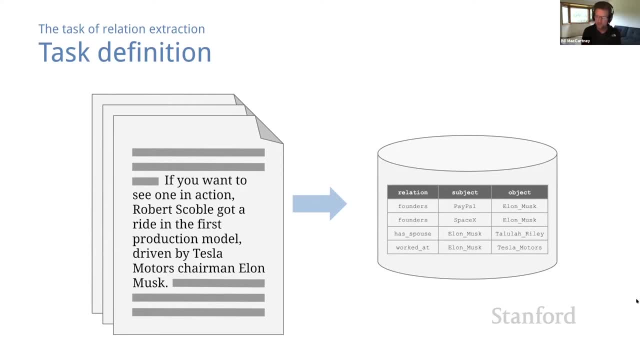 If we can accumulate a large knowledge base of relational triples, we can use it to power question answering and other applications. Building a knowledge base like this manually is slow And- I quote- expensive, But much of the knowledge that we'd like to capture is already expressed in abundant. 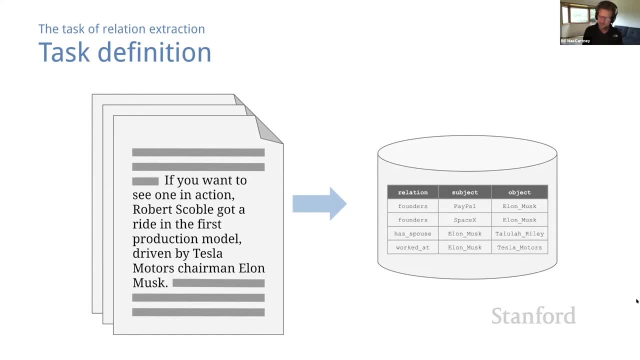 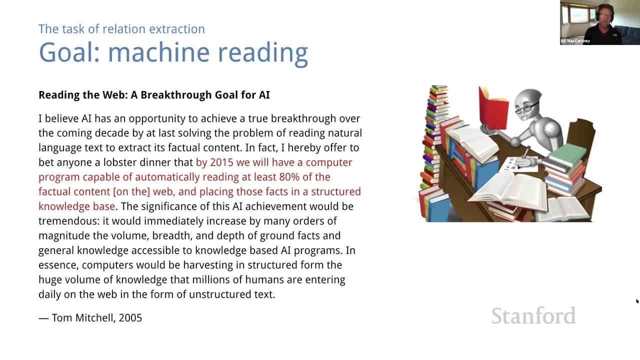 text on the web. So the aim of relation extraction is to accelerate knowledge-based construction by extracting relational triples from natural language text. Here's a nice articulation of the vision for relation extraction. This is from Tom Mitchell, who is the former chair of the machine learning department at CMU. He's also the author of one. 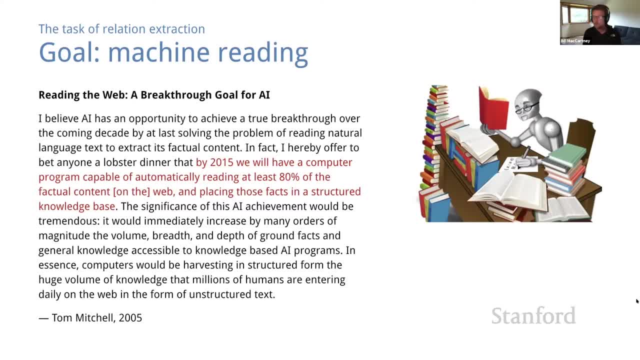 of the first textbooks on machine learning. By the way, he was also the PhD advisor of Sebastian Thrun and Oren Etzioni. He wrote this piece in 2005,, describing a vision for machine reading, And he offered to bet a lobster dinner that by 2015,, we will have a computer. 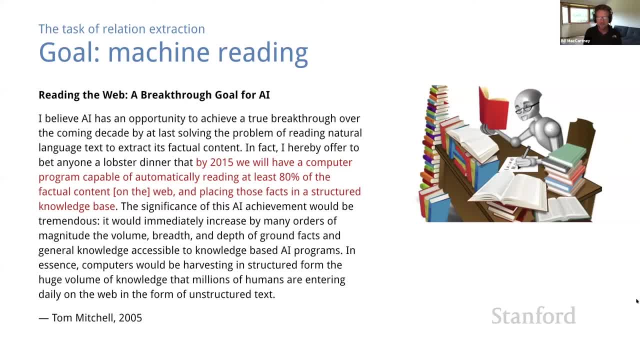 program capable of automatically reading at least 80% of the world's computer Factual content on the web and placing those facts in a structured knowledge base. I think we've come pretty close to achieving that goal, And this is exactly the goal that 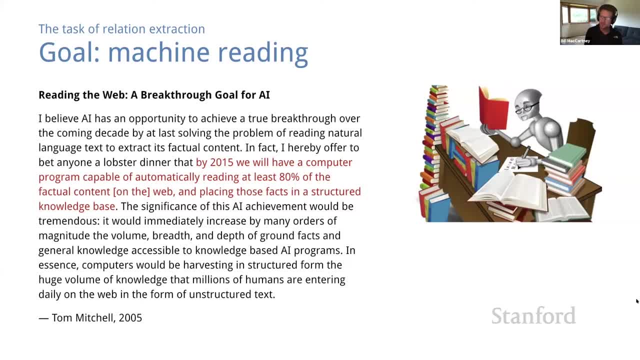 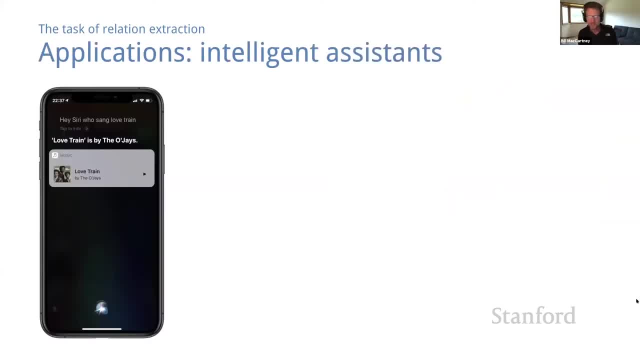 relation extraction aims at to extract structured knowledge from unstructured text. One of the things that makes relation extraction an exciting topic is the abundance of real world applications. For example, nowadays, intelligent assistants like Siri or Google can answer lots of factual questions, like who's saying love train. To do this they rely on. 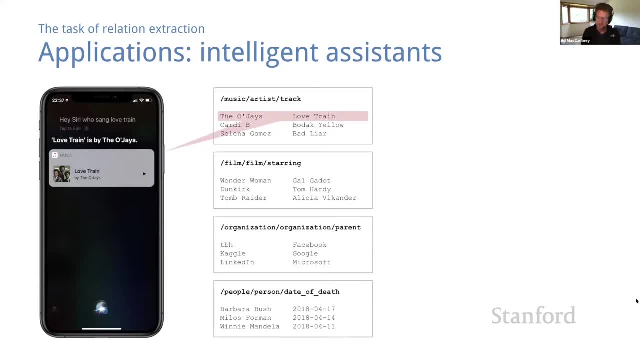 knowledge bases, or KBs, containing thousands of relations, millions of entities and billions of individual facts. There are many different strategies for building and maintaining and extending these KBs, But, considering how enormous they are and how quickly the world is creating new facts, it's a process that you want to automate as much as possible. 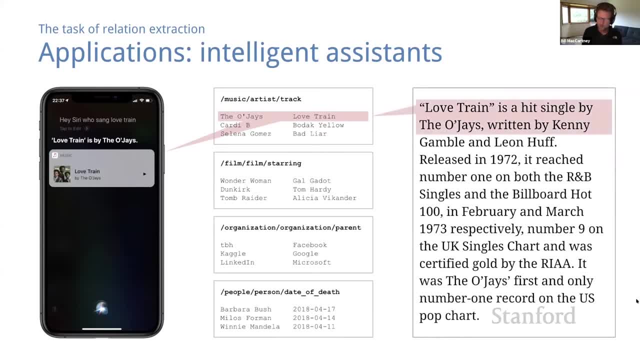 So more and more relation. extraction from the web is a is hugely strategic for Apple and Google and other companies. In fact, in 2017, Apple spent $200 million to acquire a startup called Lattice, which was co founded by Stanford professor Chris Ray, whom some of you may know specifically for. 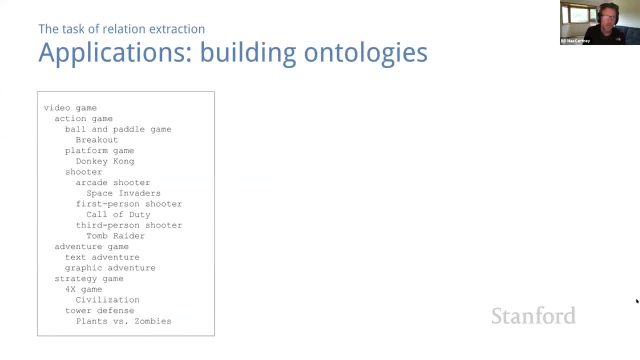 this purpose. Another example is building ontologies. If you're running an app store, you're you're going to need a taxonomy of categories of apps and which apps belong to which categories. One category of apps is video games, But if you're a gamer, you know that there are subcategories. 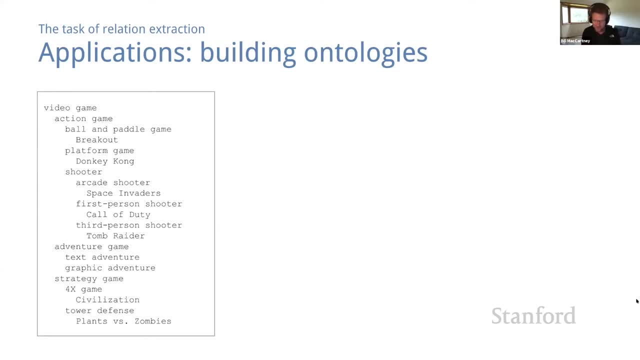 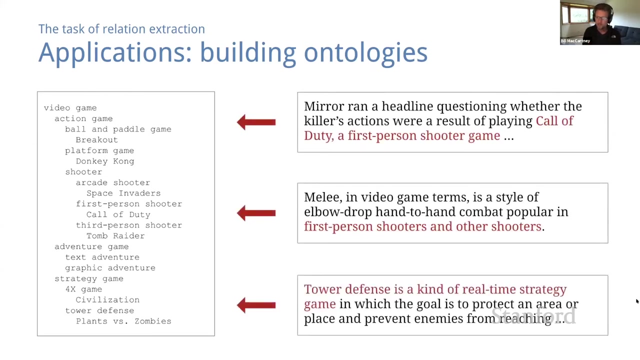 and sub-subcategories and sub-sub-subcategories of video games, And new ones keep appearing, and new games appear every day. How are you going to keep your ontology up to date? Well, there's a lot of people writing about video games on the web, So maybe relation extraction can. 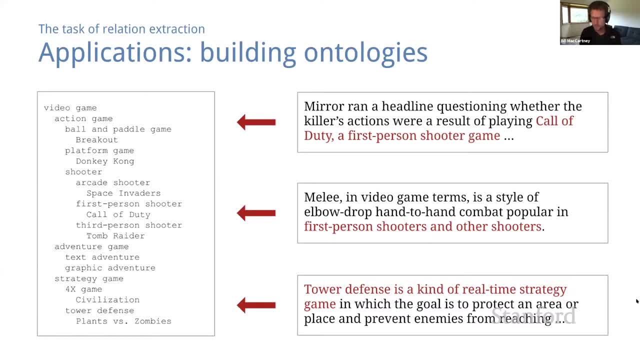 help. The relation between a category and a subcategory or between a category and an instance of the category can be a target for relation extraction, And similarly you can imagine using relation extraction to help build or maintain ontologies of car parts or companies or viruses. 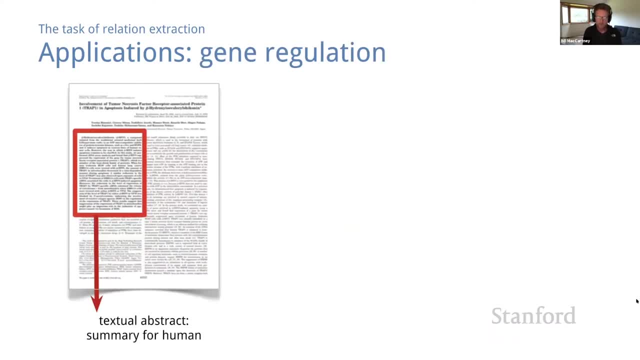 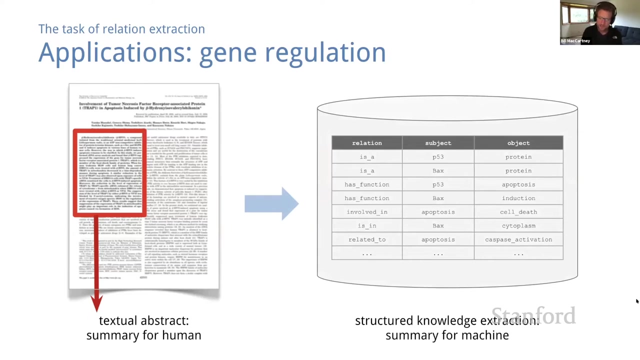 Another example comes from bioinformatics. So every year there are thousands of new research articles describing gene regulatory networks. If we can apply relation extraction to these articles to populate a database of gene regulation relationships, then we can begin to apply existing well-understood data mining techniques. We can look for statistical correlations or apply 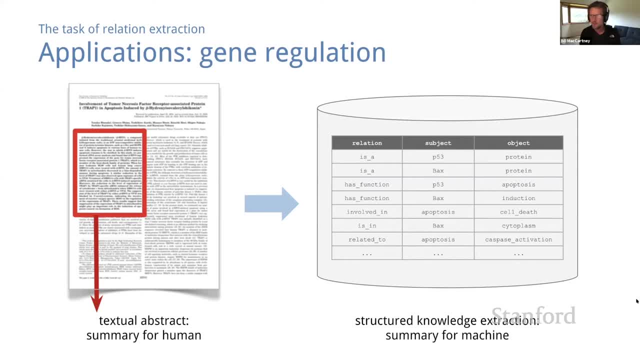 clever graph algorithms to activate them, And we can also apply statistical correlations to the identification networks. The sky's the limit. We've turned something that a machine can't understand into something that a machine can understand. So let's turn to the question of how. 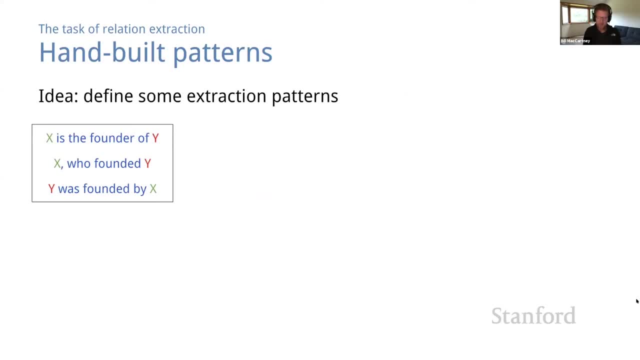 you'd actually solve this problem. The most obvious way to start is to write down a few patterns which express each relation. So, for example, if we want to find new instances of the founders relation, so we can use patterns like X is the founder of Y or X comma. who founded Y or Y comma? 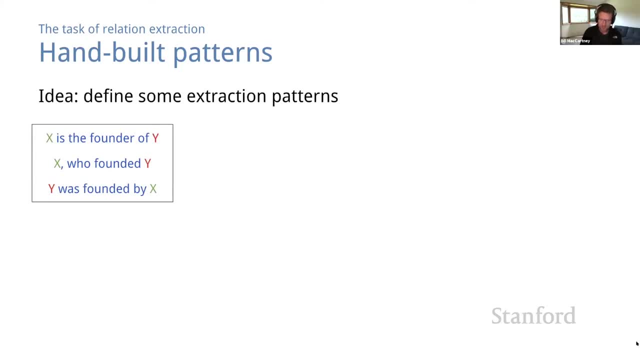 was founded by X, And then, if we search a large corpus, we may find sentences like these that match these patterns and allow us to extract the fact that Elon Musk founded SpaceX. So this seems promising, And in fact this was the dominant paradigm in relation extraction. 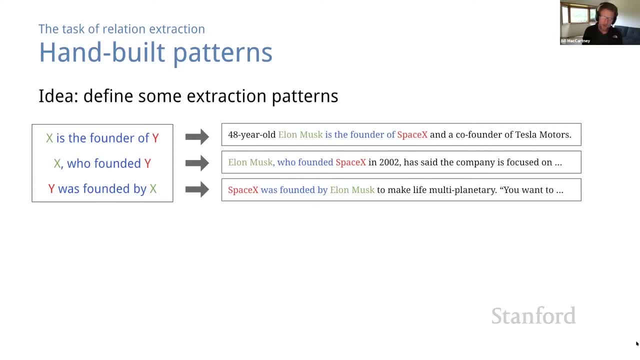 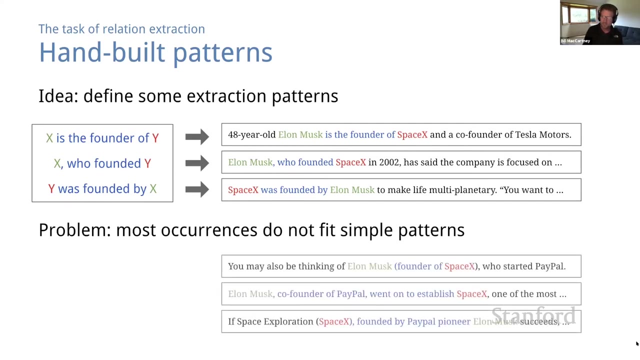 in the early days, But this approach is really limited. The central challenge of relation extraction is the fantastic diversity of language, the multitude of possible ways to express a given relation. For example, each of these sentences also expresses the fact that Elon Musk founded 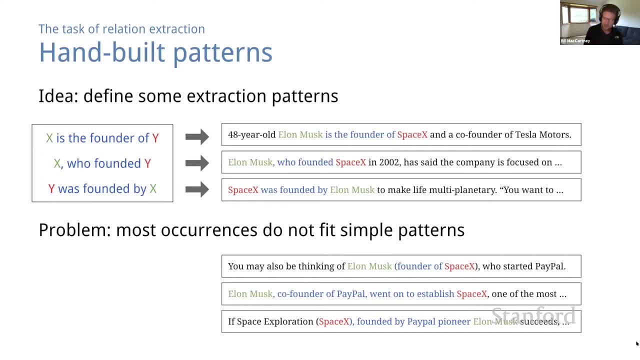 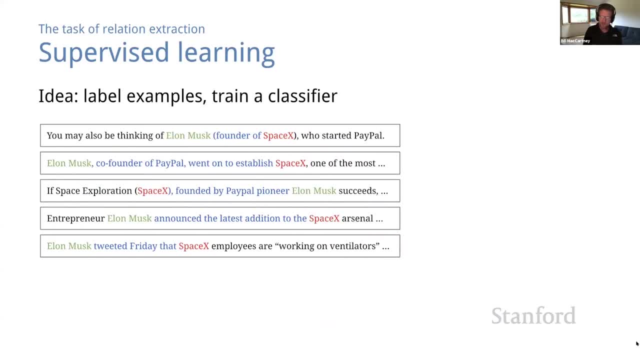 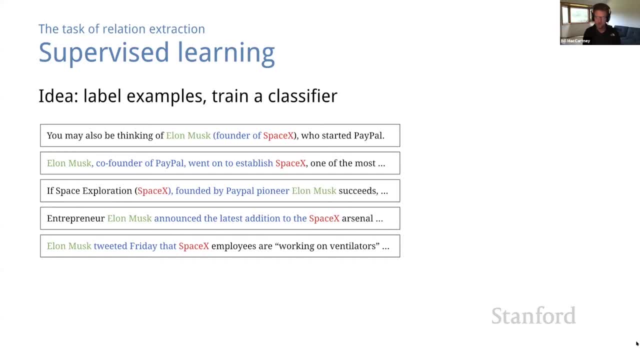 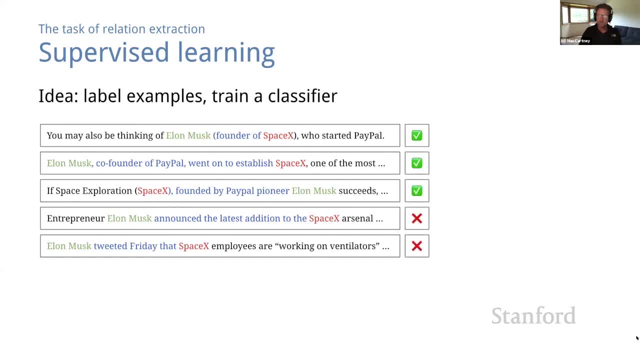 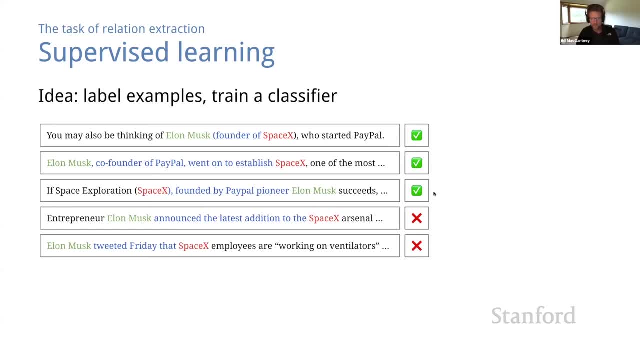 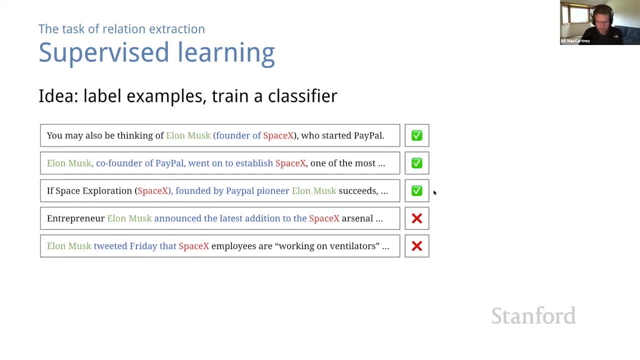 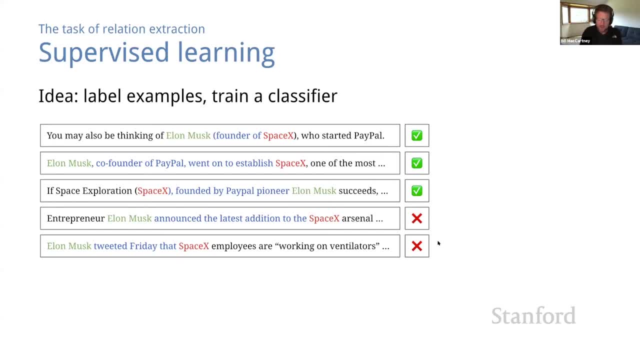 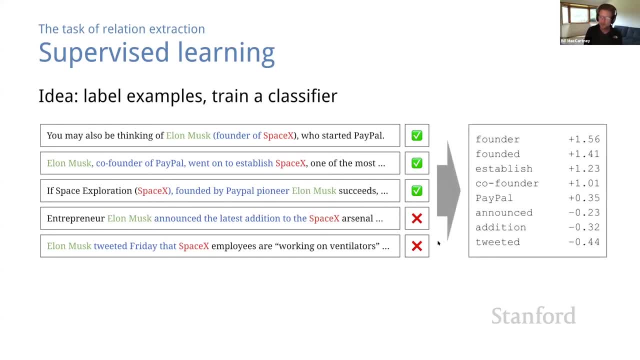 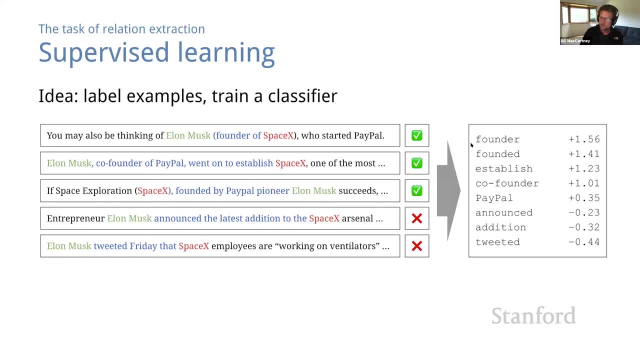 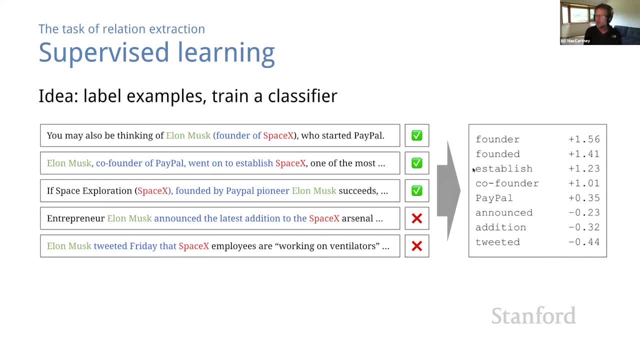 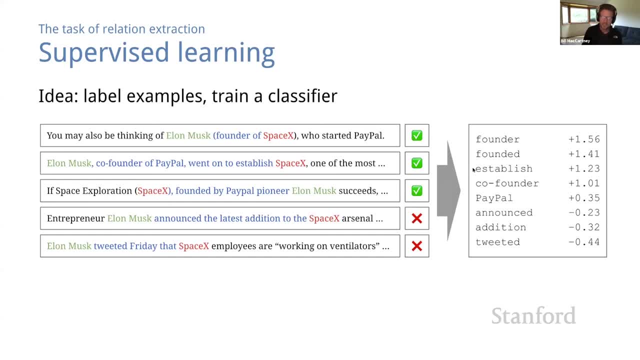 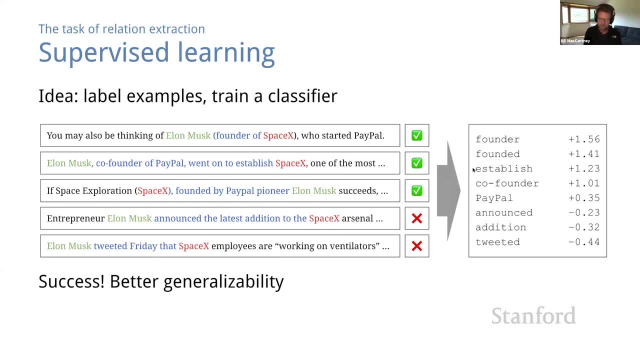 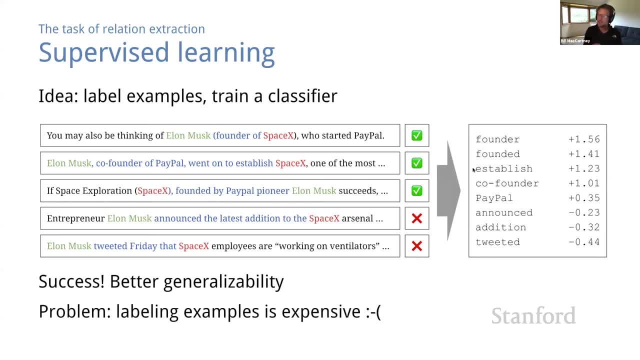 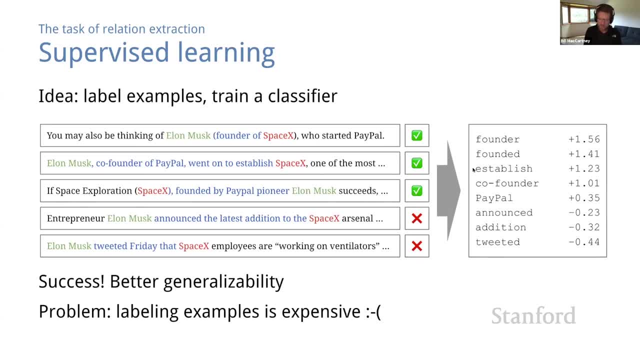 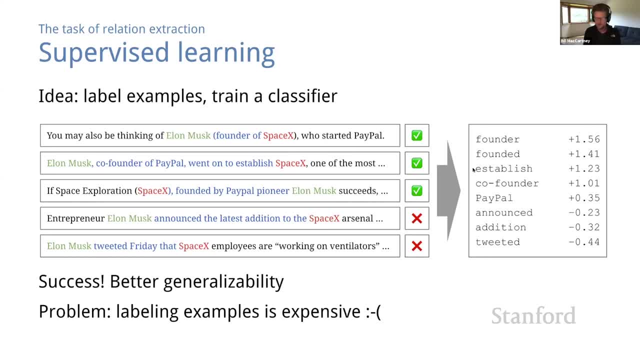 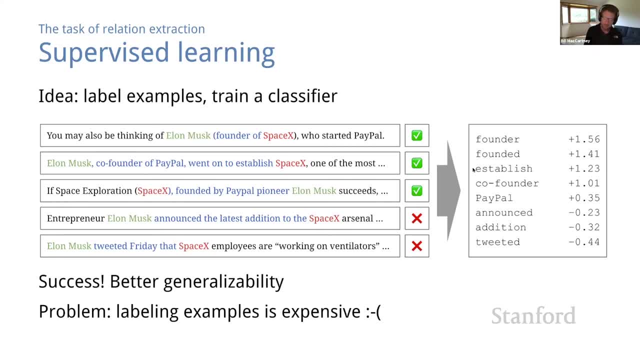 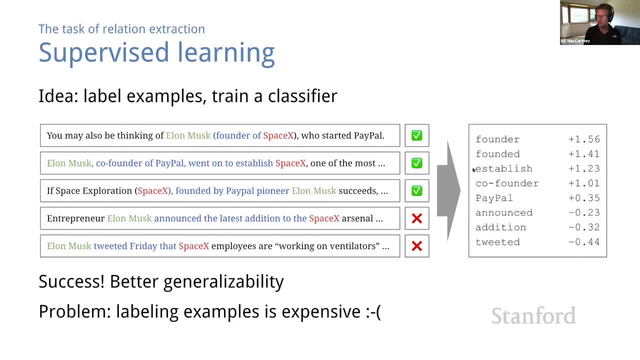 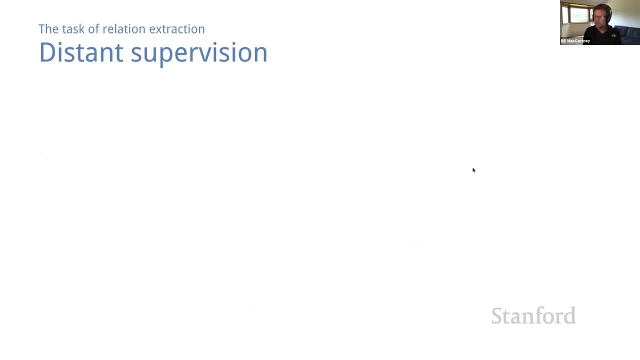 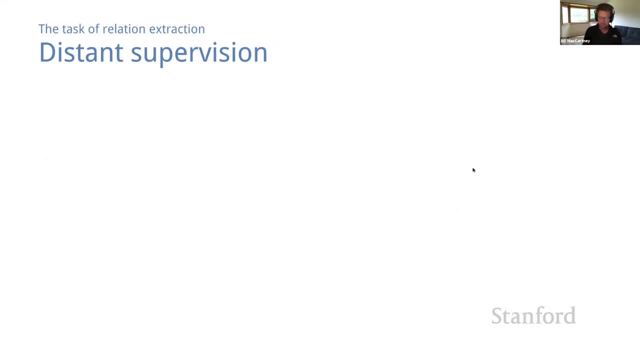 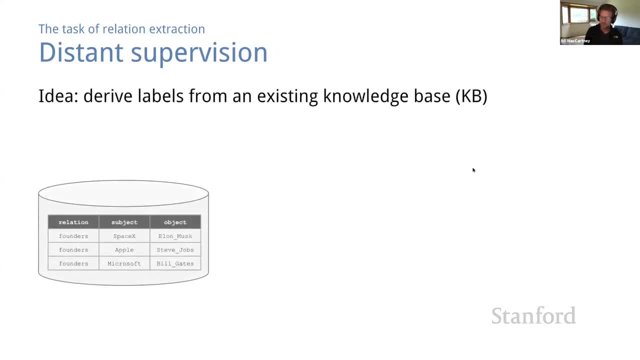 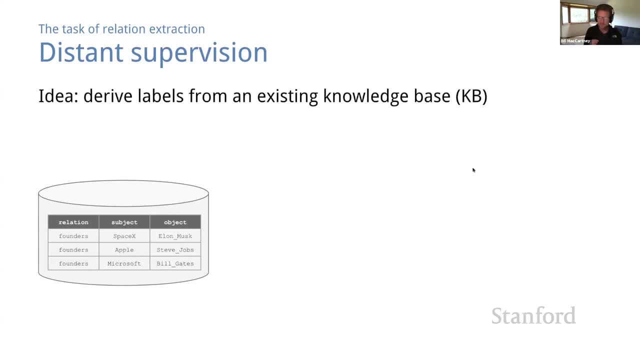 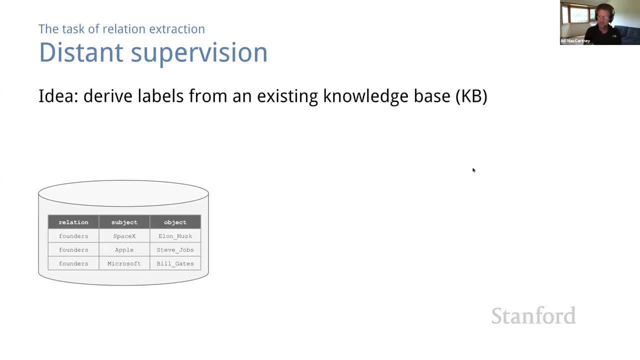 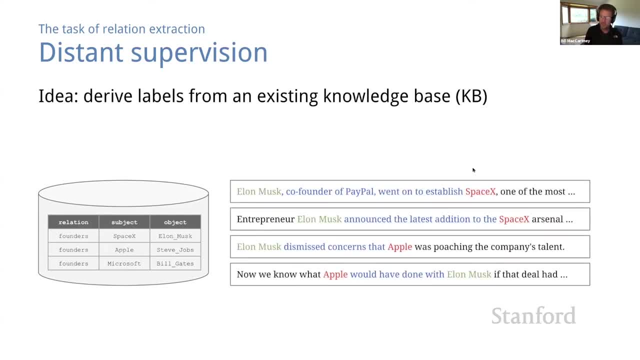 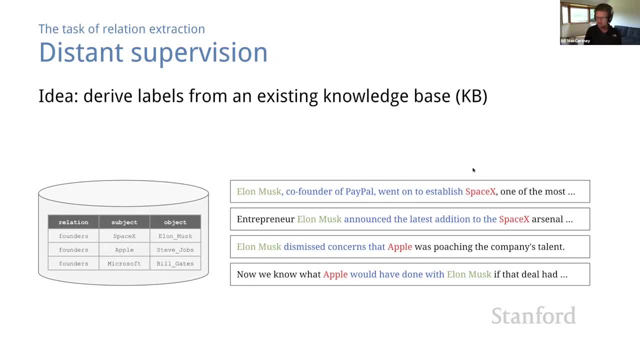 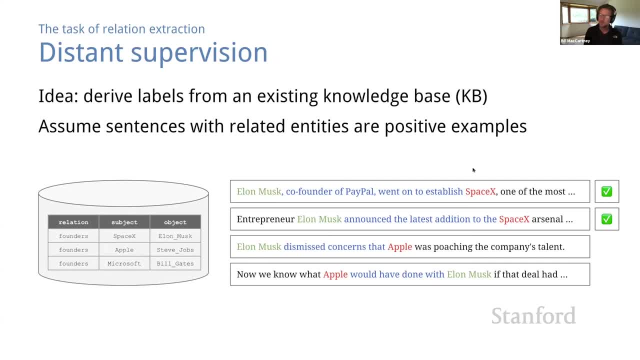 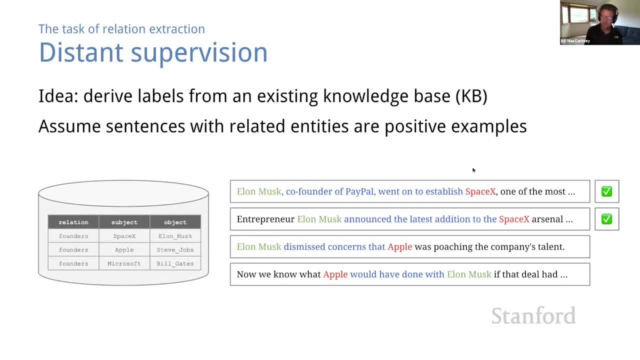 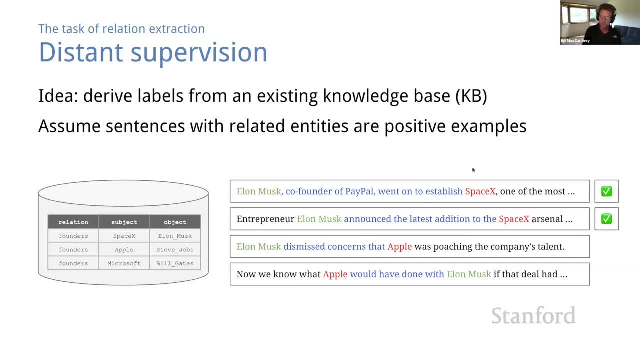 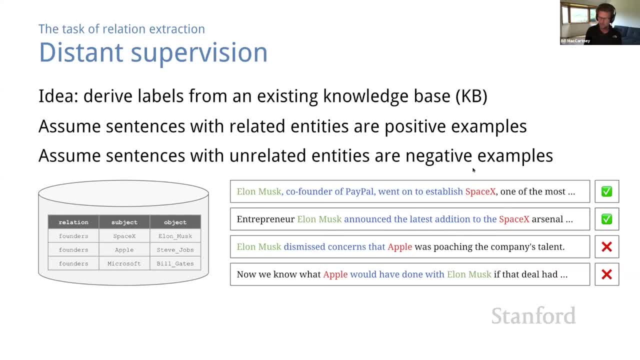 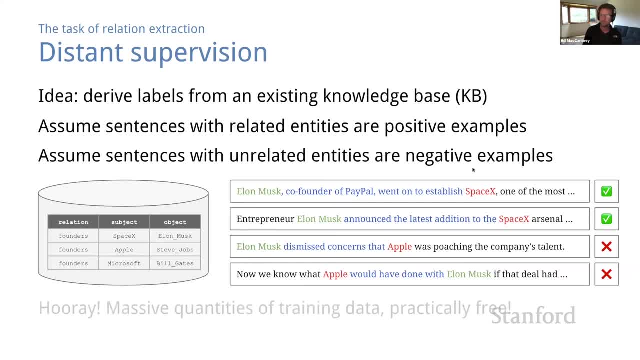 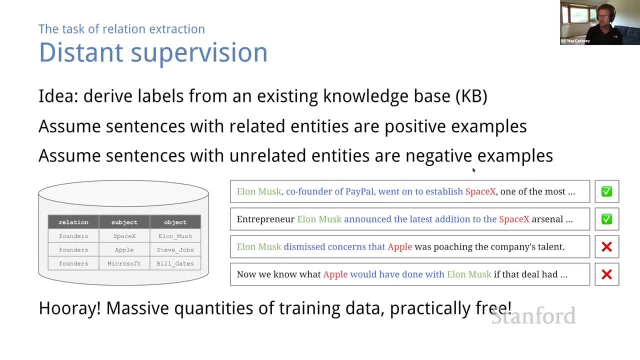 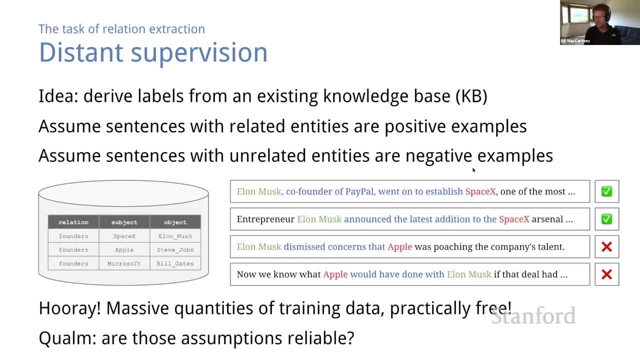 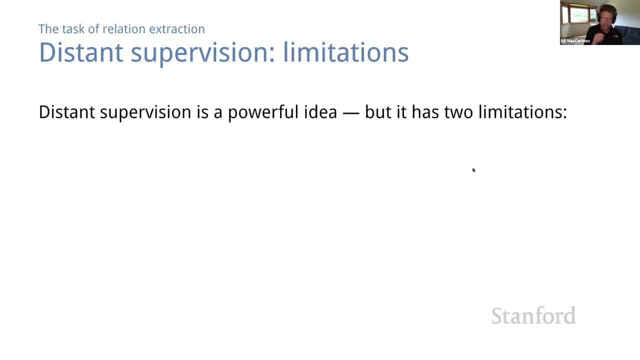 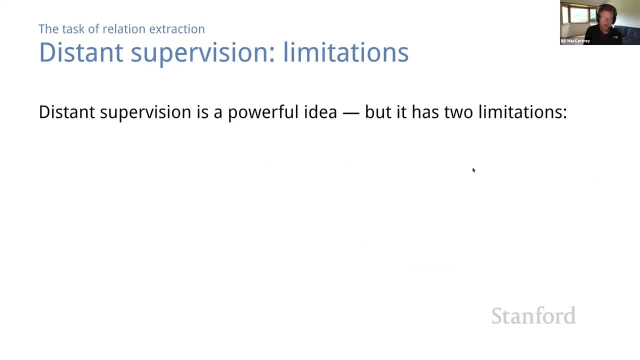 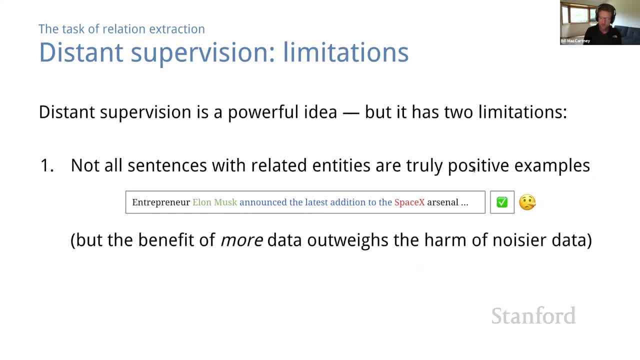 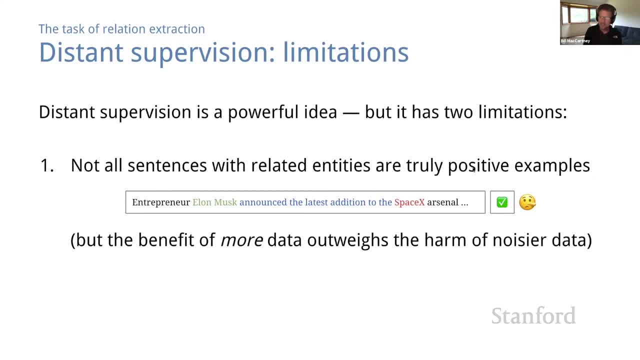 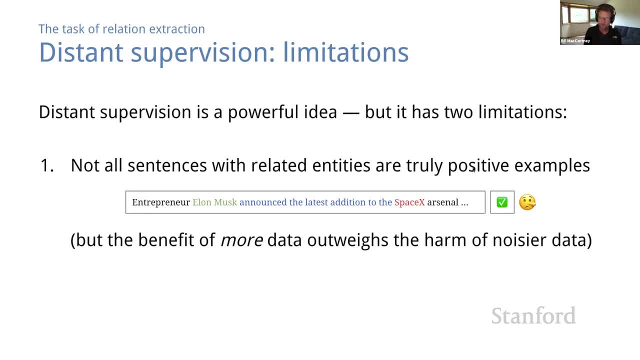 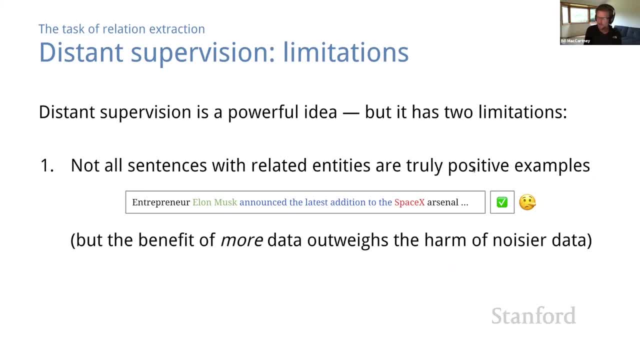 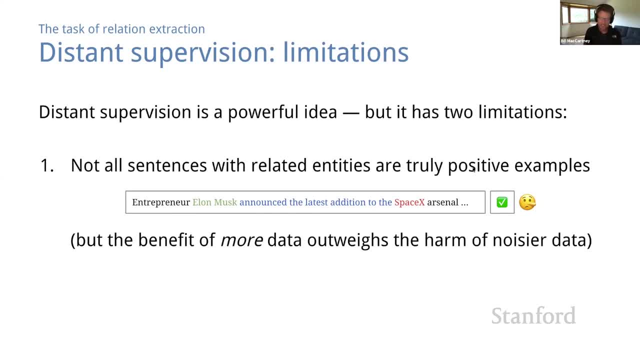 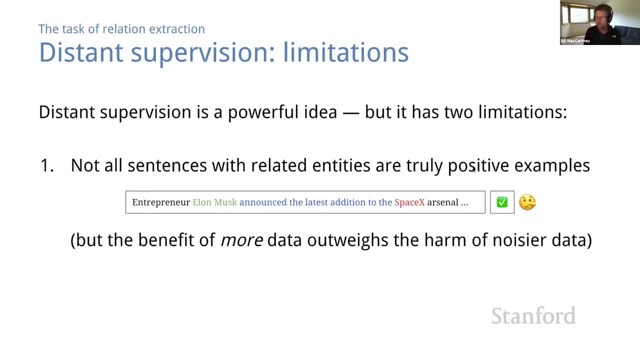 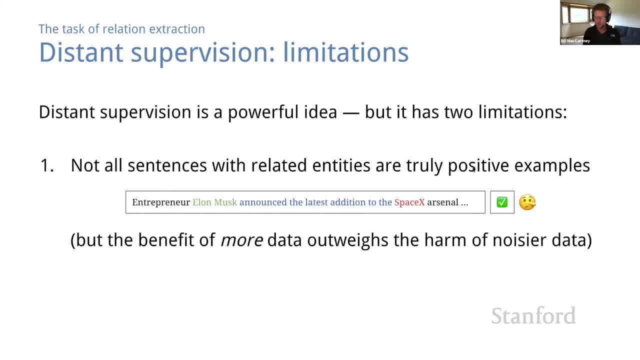 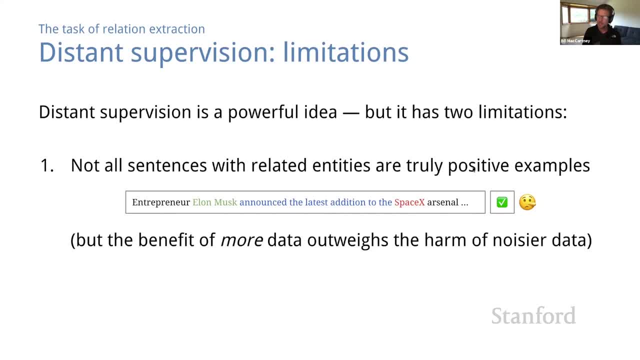 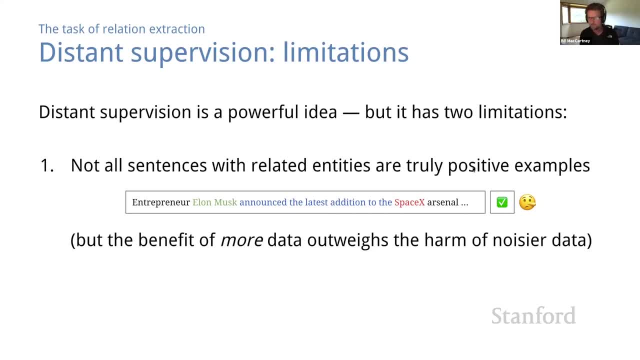 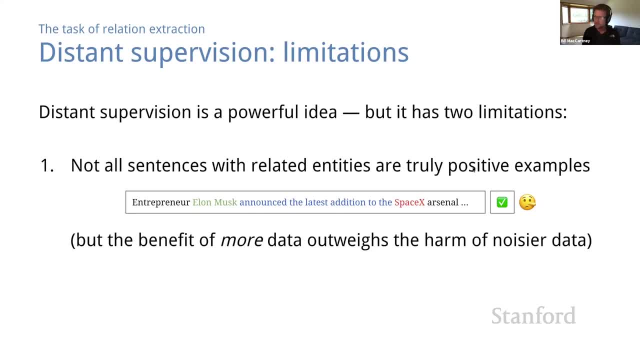 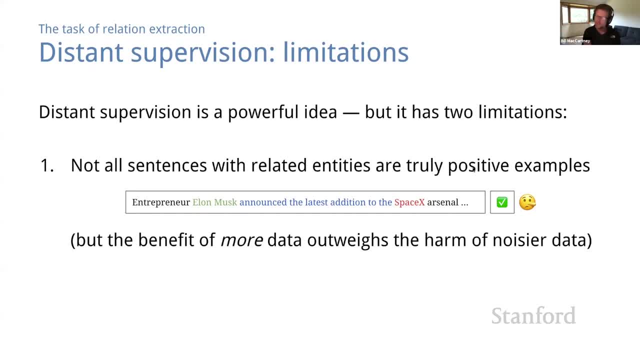